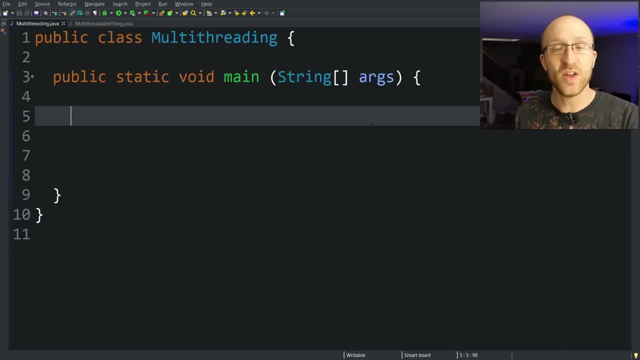 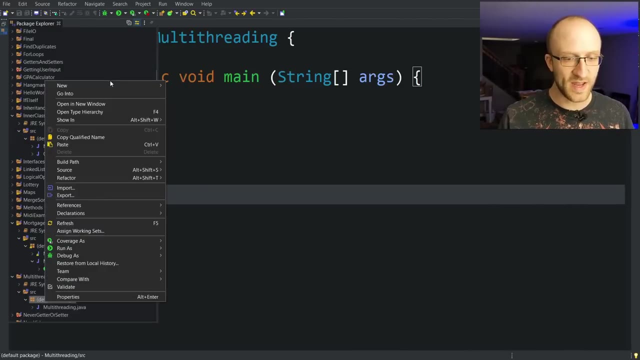 a new thread. The first way is to have a class extend the thread class. That might sound a little complicated, but it's really not. So to do that right here, next to your main class, you're just going to want to create a new Java class. You can call it whatever you want, It doesn't matter. 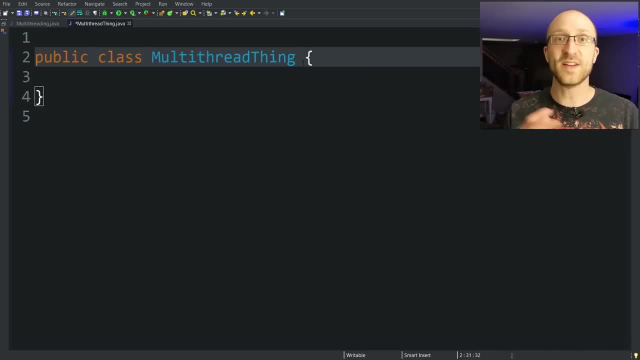 We'll call it a multithread thing. Now again, it doesn't matter what this is called, but it does have to extend threads. So now that this class extends thread, the only other thing you have to do in this class to make- 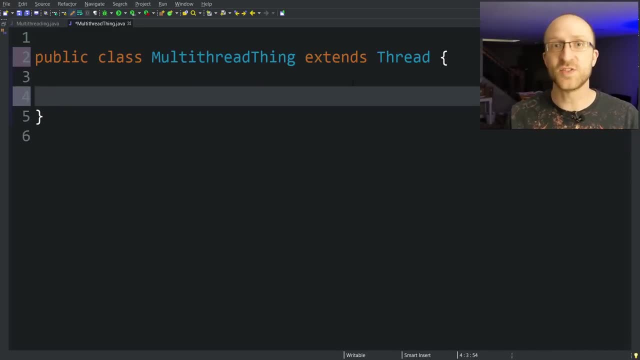 it multithreadable is to override the thread classes run method. To do that you just have to type in public void run open, close parentheses and then open and close curly braces. Since we're overriding the thread classes run method here, it's good practice to put in an at override. 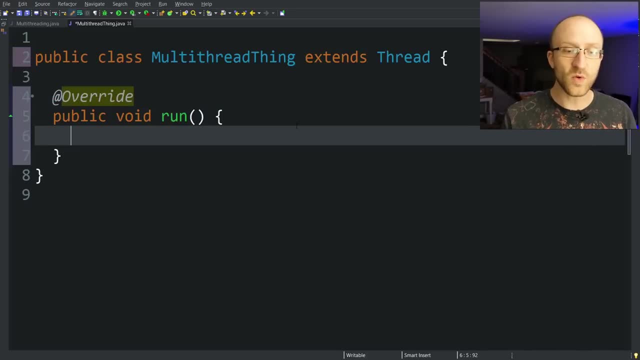 annotation here above it. So that's really all the setup that you need. The only thing you have to do now is write whatever code that you want to run in multiple threads. So that's really all the setup that you need. The only thing you have to do now is write whatever code that you want- Coffee. 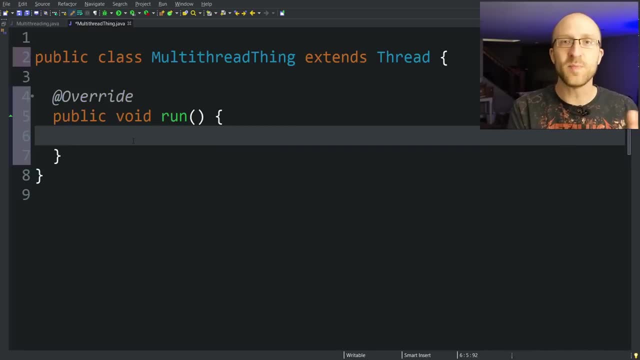 machine is going to give you inside this run method. Let's just do something really simple here, like count up the numbers from one to five. So we can just do that with a simple for loop. for int i equals one, i less than or equal to five plus plus. System. dot out print line i. 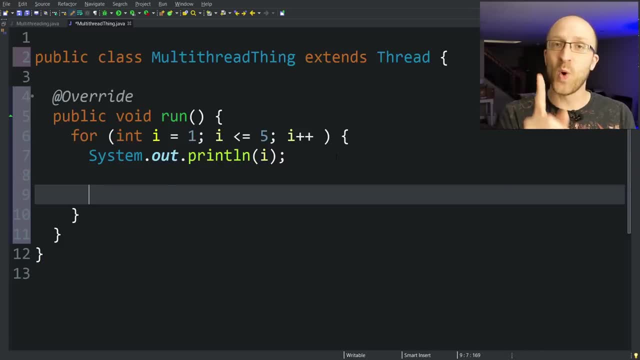 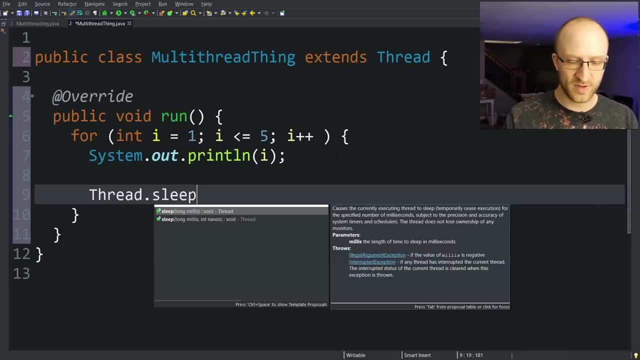 and just to make this a little bit more interesting, We're going to make it a sleep for one second between each number it prints out. That way we can watch it print out each number one at a time. To do that we can just do thread dot, sleep And we put in the number of the. 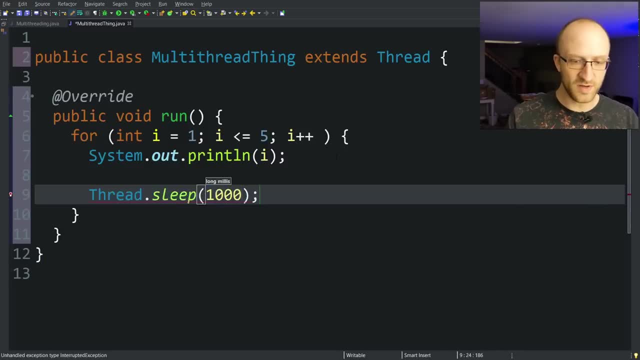 needle, but it says baby in front And what we'll see that does is the screen gets a little bit more of milliseconds. we want it to sleep, so that can be a thousand thousand milliseconds is one second. eclipse is giving us an error here because we have to surround a threadsleep with a try catch. 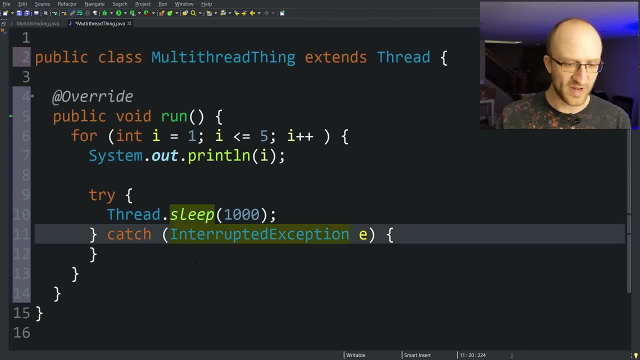 so we can just have it automatically do that. we don't have to do anything special if we run to any exceptions, so this empty catch block is just fine. so now we have a class that extends thread and we have overridden the thread classes run method. so now how do we go about actually? 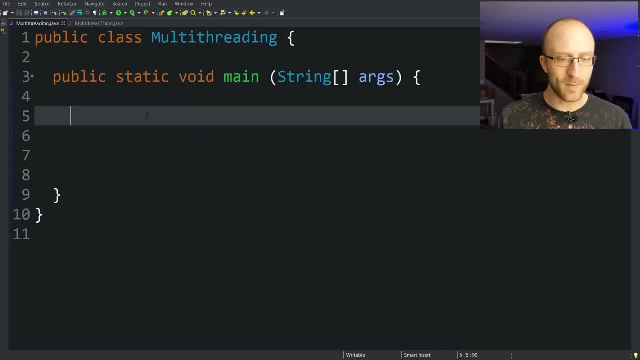 kicking off this code in multiple threads. to do that, let's go back to our main class and first create an object of that multi-thread thing class that we created, let's call it: my thing equals new multi-thread thing. now we have this my thing object, and you and you might think, since we 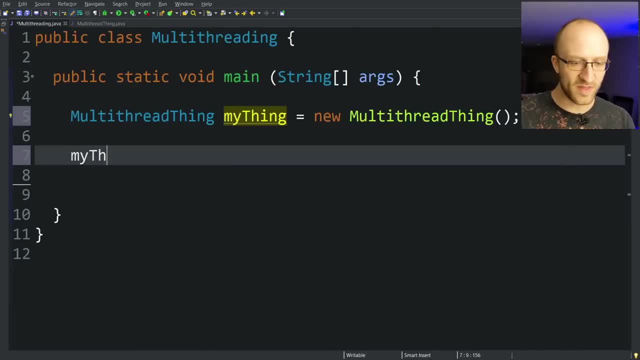 implemented the run method that we want to actually call my thing dot run. now you can do that. that'll work. it'll run the code that we wrote in that run method, but it won't actually do it in a separate thread. to actually kick off a new thread, you have to instead call my thing dot. 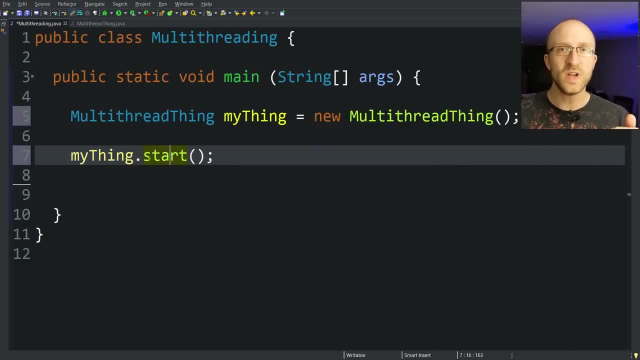 start. so now what'll happen here? as soon as it gets to that, this part in the code, java will branch off a brand new thread and start running this run method, and after it kicks off that new thread and lets it go do its thing, it'll proceed down the main thread. 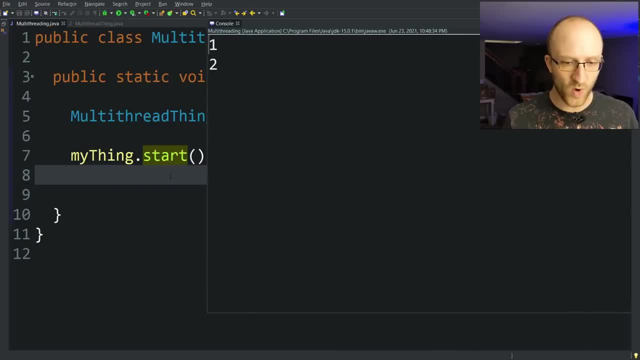 that it was executing here. so now we can go ahead and run it and watch it go with just one thread: one, two, three, four, five and then the program finishes. so that's cool and all. but the whole point of this is multi-threading. so let's go ahead and create a second thread and watch them go at. 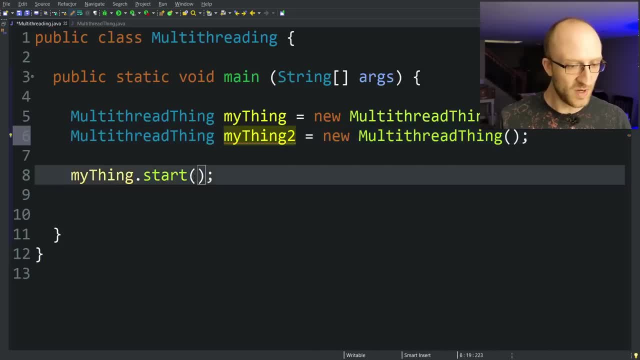 the same time. so let's just copy paste that, we'll say my thing 2, and then copy paste that and say my thing 2: dot start right after the first. my thing now: if we run our program, we can truly see that we have two different threads counting up one to five at exactly the same time as a quick note. if we 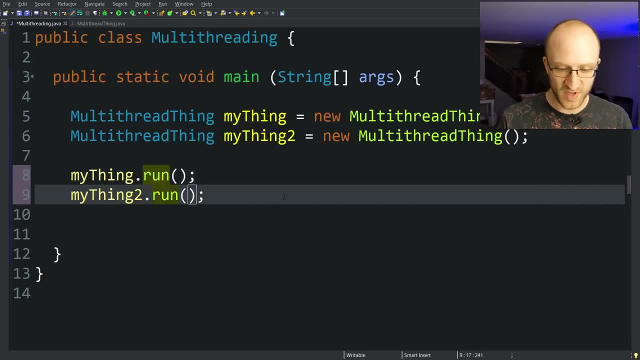 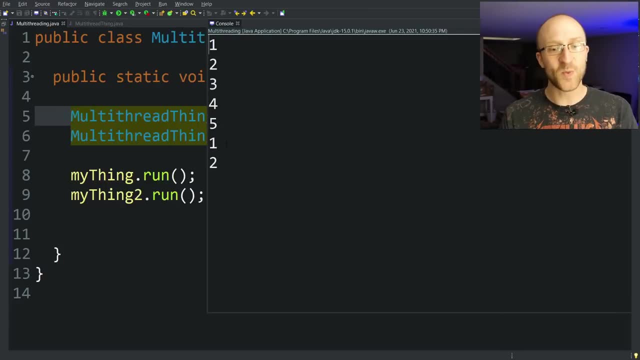 would have called our run method. instead, let's go ahead and change these both to use run. we can see that it's not actually doing multiple threads. it's doing the first- my things run, printing out one through five and then, once that's done, it finishes and does the second things, a counting of one. 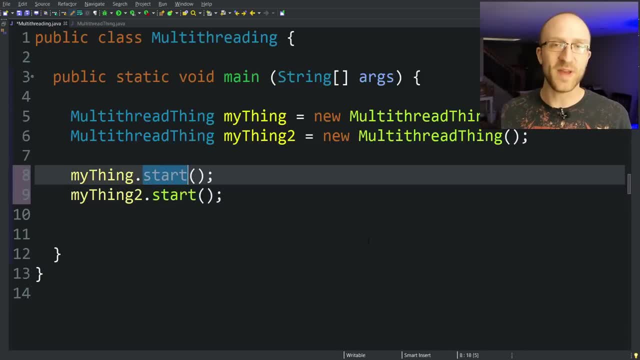 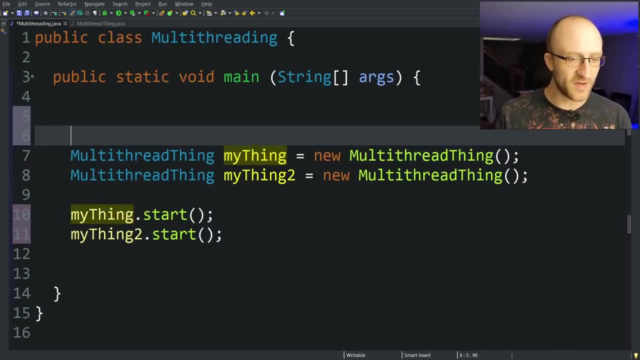 through five. it's not doing them both at the same time. so remember, you have to use the start method if you want to run multiple threads at the same time. if you want to run multiple threads at the same time. if you want to run multiple threads at the same time, you really want multiple concurrent. 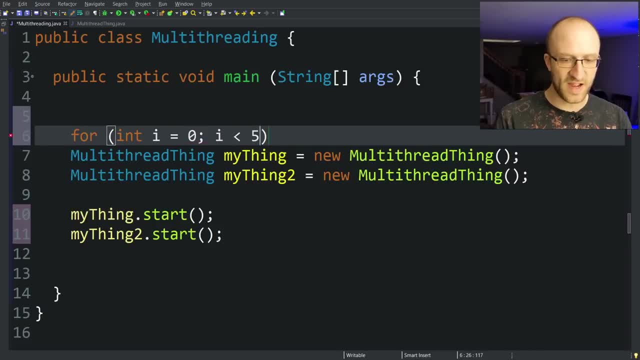 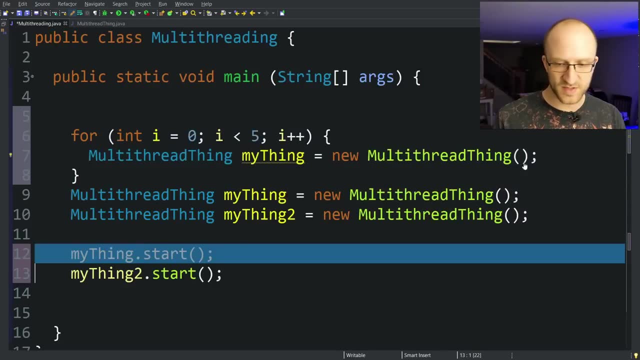 threads. and now, if you want more than just like two threads like this, you can create a whole bunch of them very easily by doing something like a for loop or: and i equals zero, i less than five. let's say we want to try doing five threads at a time, i plus plus. we can just take this line, copy it in: 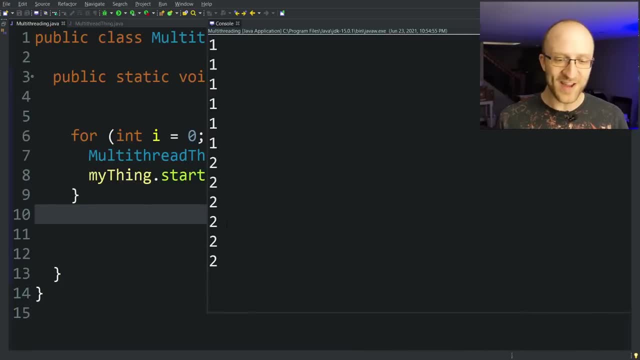 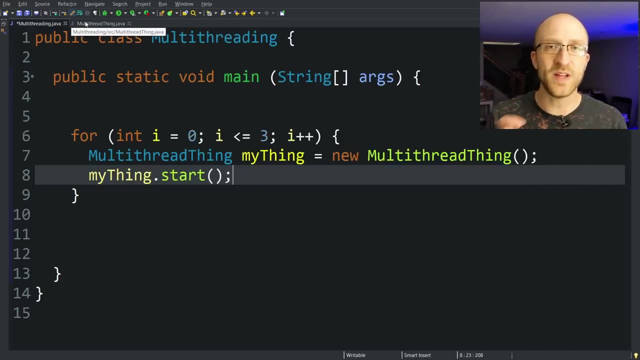 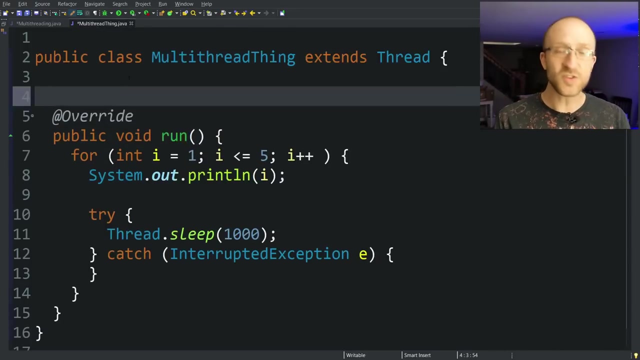 here and the start command here. get rid of all this. we don't need it anymore. and now we'll create, and you can create- multiple threads. let's say we want to do it at the same time. so we give this the variable alt preview option. we get it here. slash one, root four, Ariel, delete guardians thing one. 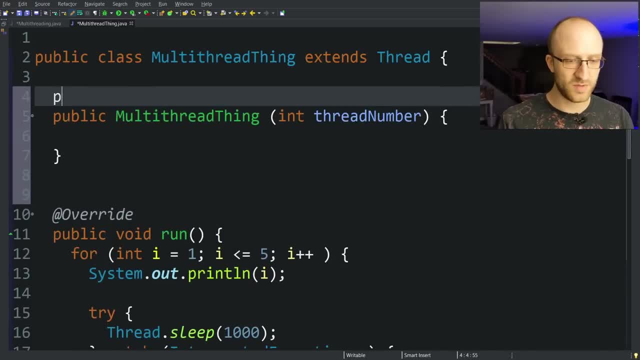 symbol we're going to say we're going to save this Singularity as one single thread thing. here we have mano and we нед malo, and below our file we're goingto have our 365 at exactly the be equal to the thread number that's passed in in the method here. So now back here in our main. 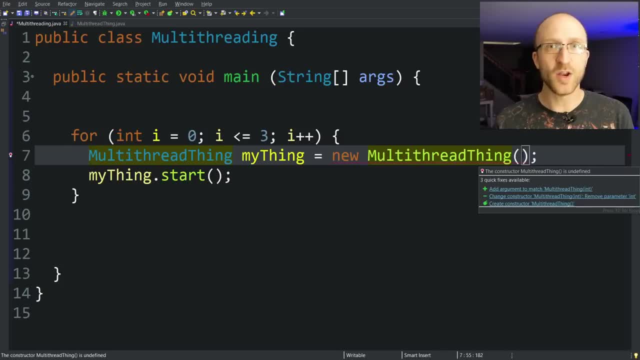 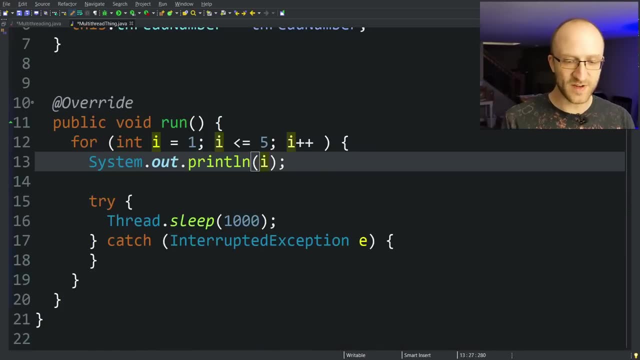 class where we're creating this multi-thread thing object, we need to pass in a number for the thread number, and here we can just use i, because we're going through a for loop anyway. But what's neat about that is, in our run method, instead of just printing out i, we can print out which thread it. 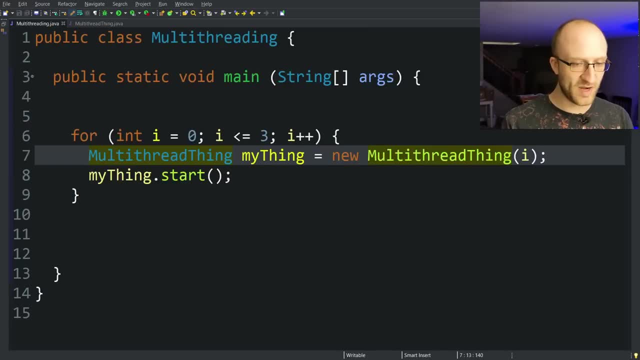 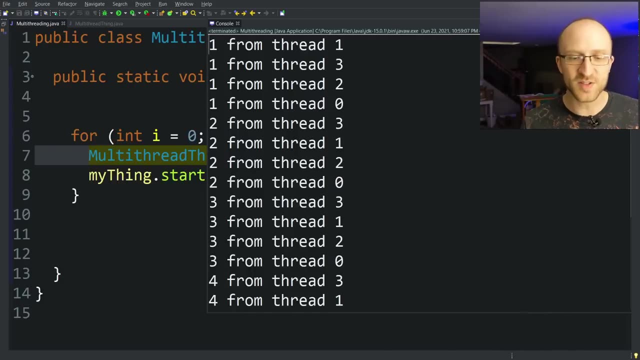 is So like from thread thread number and go back and run our program, we can now see which thread is printing which number and we get some kind of interesting results. So you might assume that because thread zero is created first, that it would get printed out first, but it doesn't In this case. 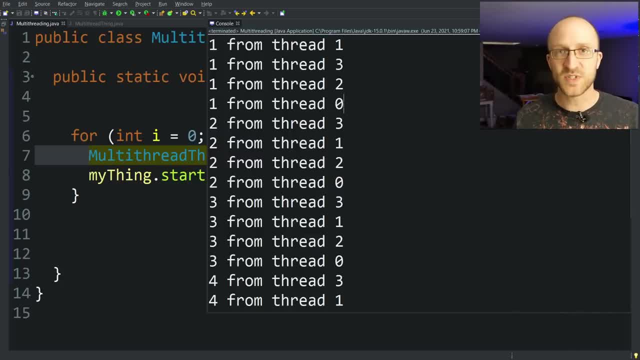 thread one happens to be printed first, and then three and then two. What that tells you is that when you break into multiple threads, there's absolutely no guarantee which thread is going to be doing its thing first. They're all running at the same time, completely independently. so there is. 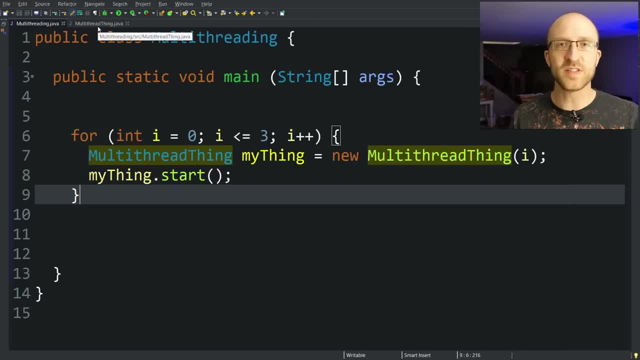 going to be some slight variance in their timing. One of the really cool things about multi-threading is that if one of the threads blows up with some kind of exception, it doesn't impact any of the other ones. All the other ones just keep going business. 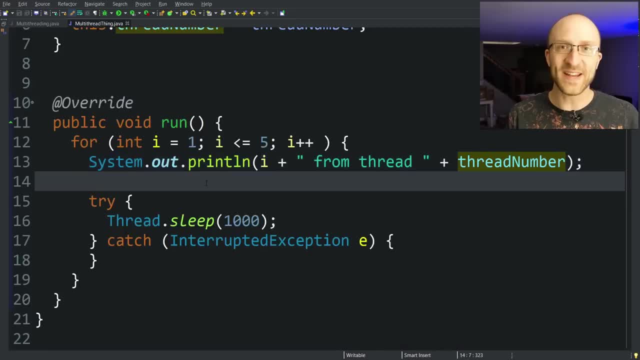 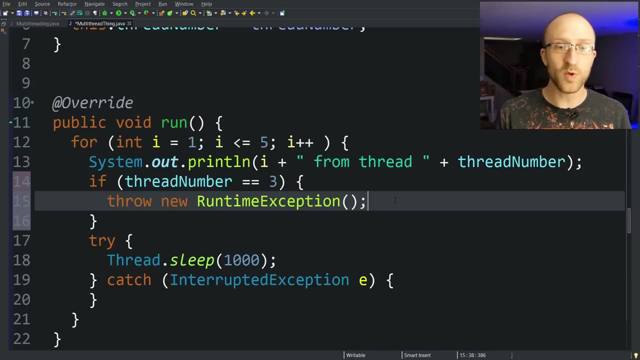 As usual. so to demonstrate that let's actually make an exception happen in one of the threads. So let's just say here in our run method we could just say, if thread number equals three, we're just going to flat out throw a new runtime exception. So of course this will make thread 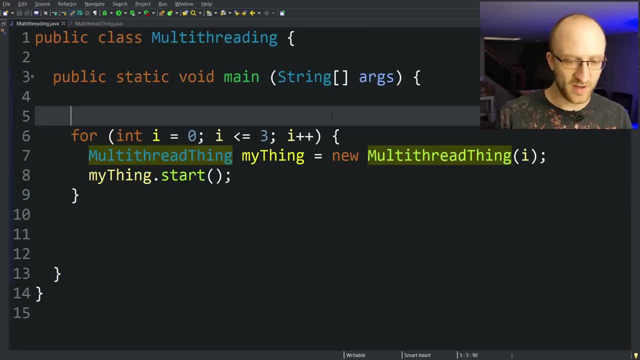 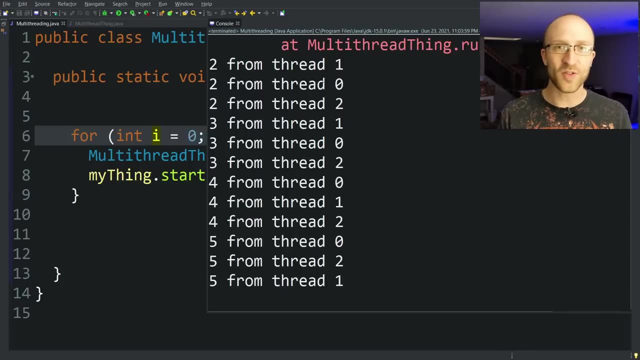 number three blow up. So now we can save that, go back and run it and we can see that thread number three blows up with a runtime exception after it prints the number one, but all the other threads go ahead and continue printing out all their numbers. Let's go ahead and get rid of that. 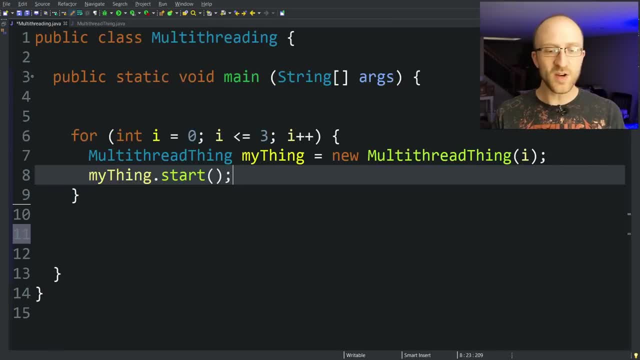 of that bit of craziness, but that even applies to our main thread. If in here we go ahead and start all these other threads counting one through five and then immediately run into an exception, that won't stop all the other threads from still completing. So if here we say, throw new. 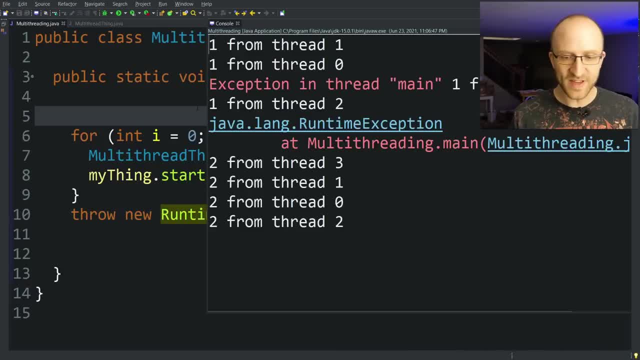 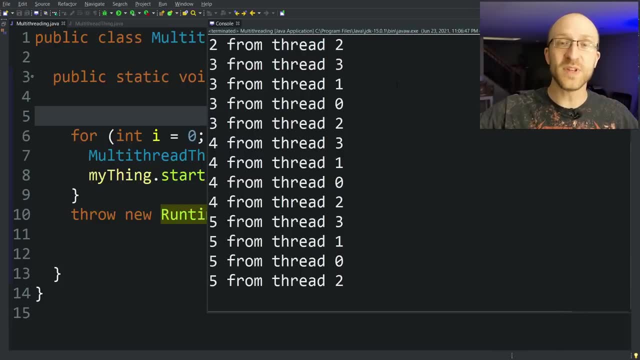 runtime exception run our program and we can see that even though we run into a runtime exception in the main thread, in our main method, all of those other threads that we kicked off continue to run completely independently because there was no exception in those threads. Now I mentioned there. 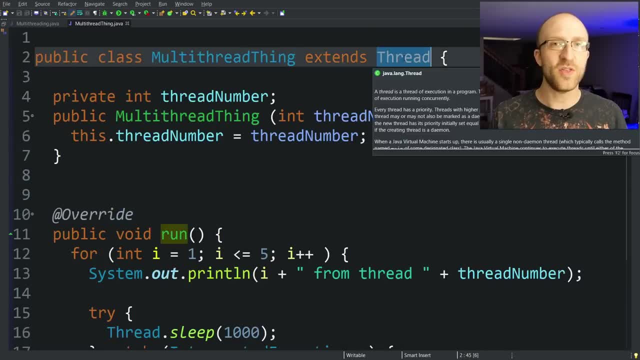 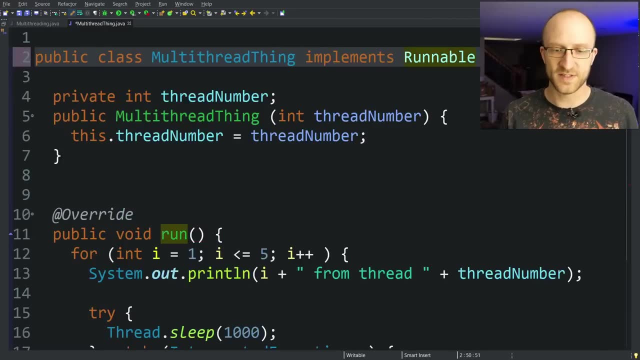 was no exception in the runable Java class, and the first way was extending the thread class, And the other way, instead of extending the thread class, you can implement the runnable interface. What's nice about that is that when you implement the runnable interface, the only thing you have to 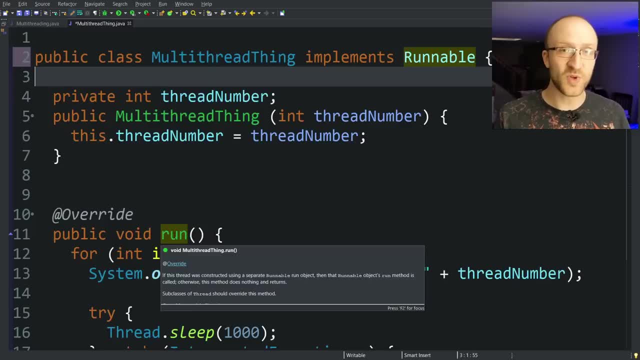 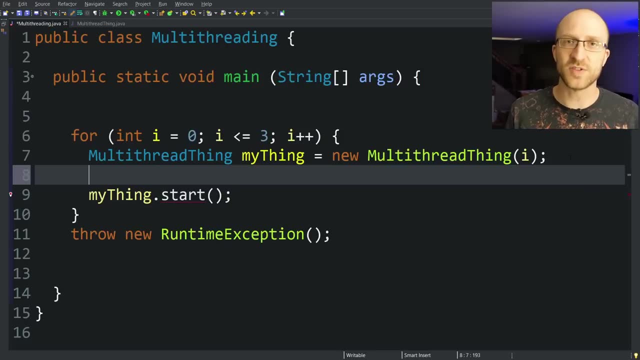 do is have your own implementation of the run method, which is the same as if you extend thread. So there's really nothing else you have to change about this class. But back here in our main method, we can't just call start anymore because we don't extend thread, so there's a small extra step, All. 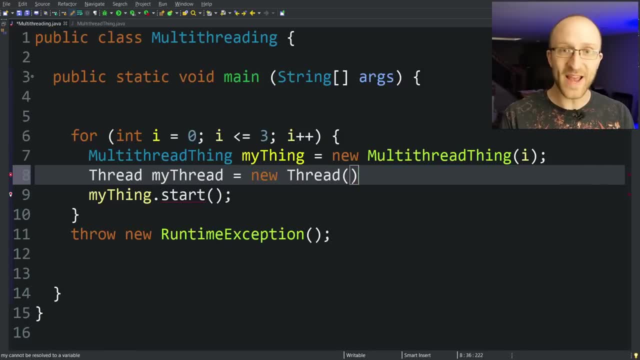 we have to do is say thread my thread, new thread and then pass it that object that implements the runnable interface. So for us it's my thing. and then instead of my thing dot start, we'll say my thread dot start. We'll also get rid of this silly exception. but really that's the only other thing that changes. You can go. 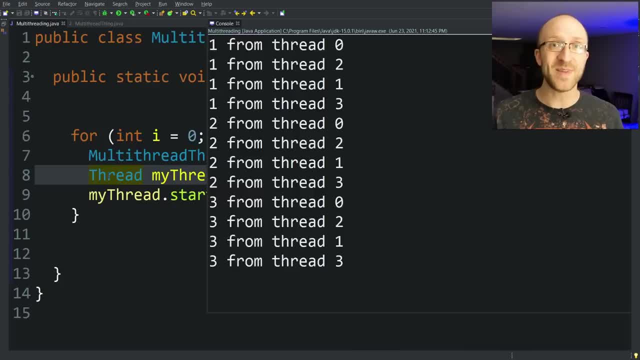 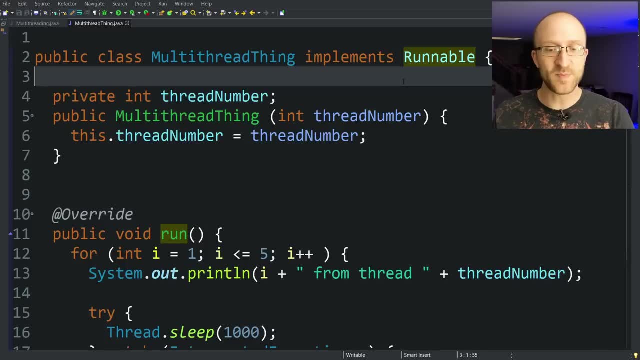 ahead and run your program, and all of your threads will operate at the same time, exactly as they did before. So you're probably wondering you know which is better. which one should I do? You can either extend the thread class, like we did first, or implement the runnable interface, like we have. 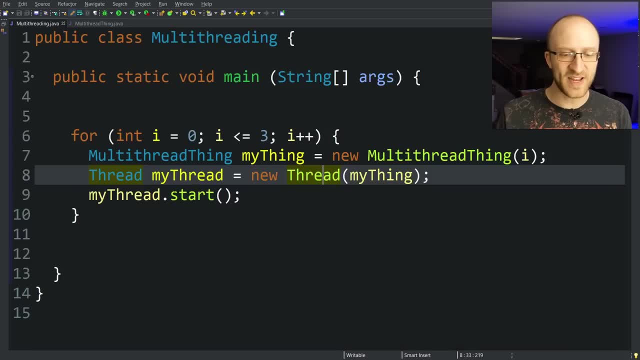 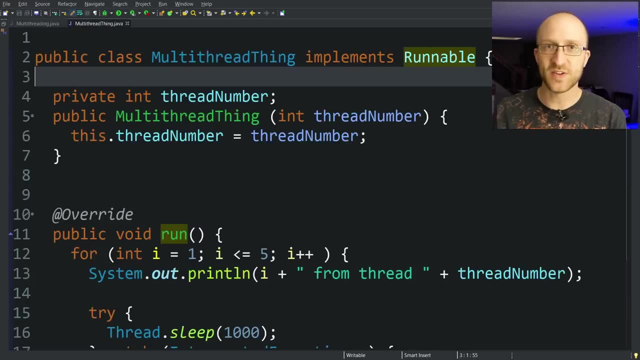 here. On one hand, if you extend the thread class, you get rid of the need to have this little extra line where you're creating a thread, but on the other hand, I think there is a major advantage to implementing the runnable interface instead of extending thread. So the problem here is that 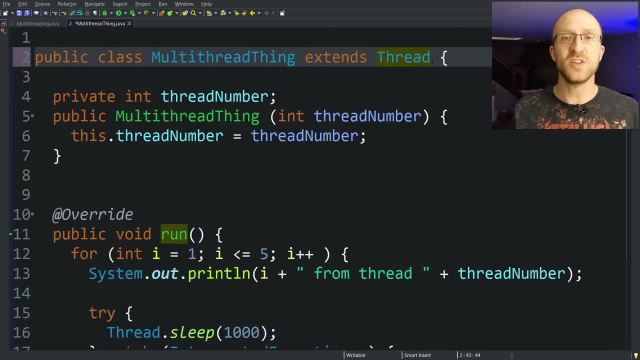 if you extend thread, you can't extend any other class. Java doesn't allow multiple inheritance. You can only be a subclass of one class, and if you are a subclass of thread by extending thread, you can't be a subclass of any other class and you're just kind of stuck. 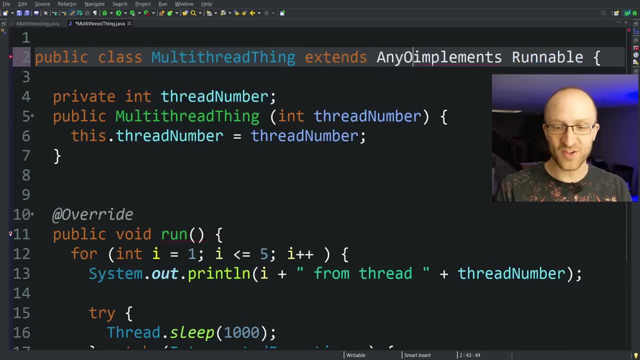 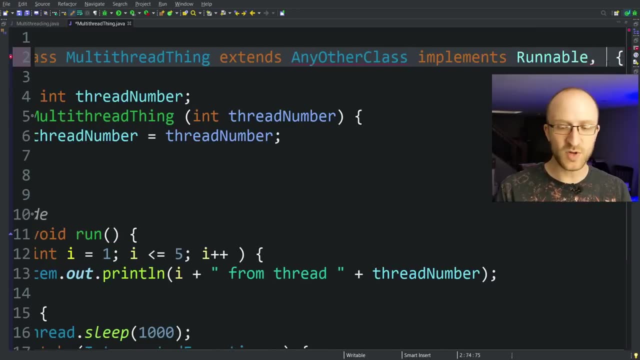 If you implement runnable, you can still have it extend any other class that you might feel a like. extending. that makes sense for your code and also Java doesn't limit the number of interfaces you can implement, so you can implement another interface here too. So, although using implements, 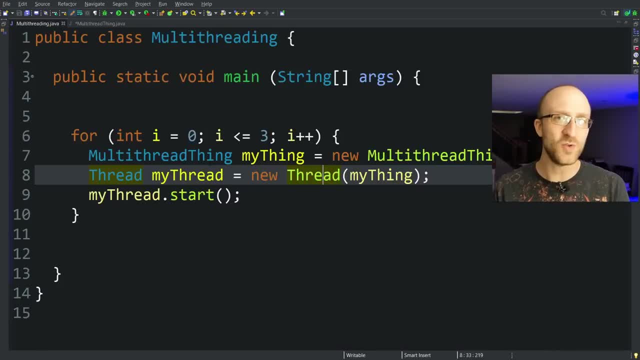 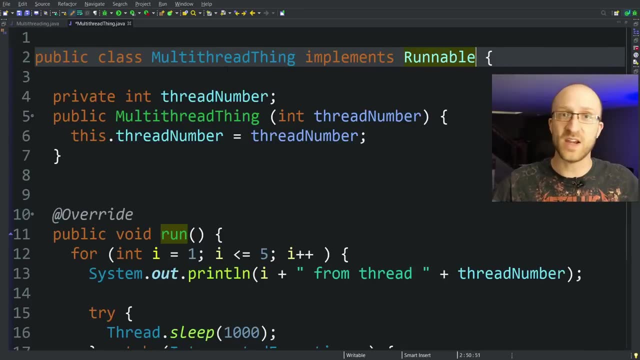 runnable kind of gives you that extra step of having to create a new thread here before you can use it. it does give you a whole lot of flexibility to be able to have your multi-threading class extend any other class you might want. There are also a few really useful methods on thread.